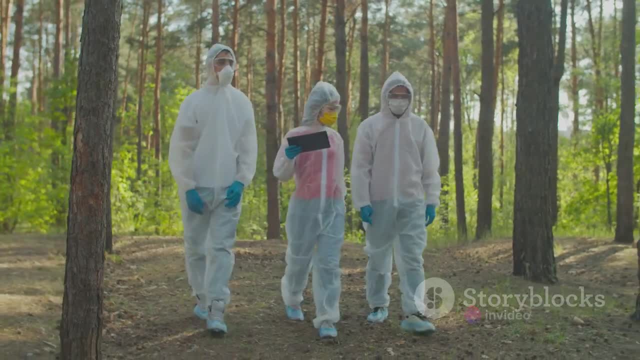 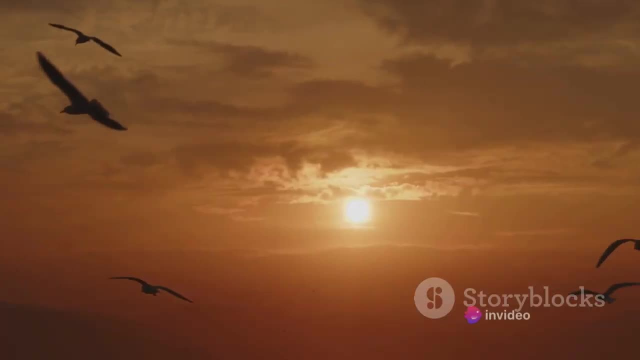 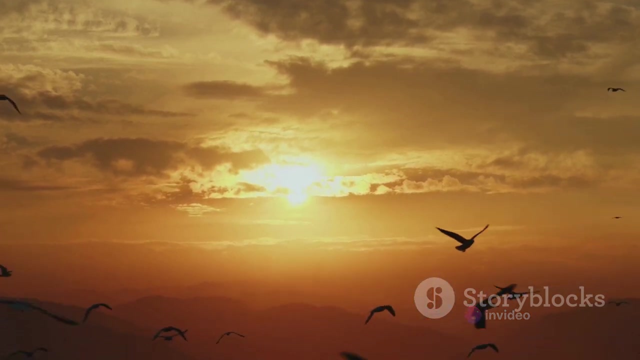 Birds, often considered environmental sentinels due to their sensitivity to changes, have been at the forefront of such studies. Recent research has unearthed some fascinating findings. Contrary to the popular belief that radiation is universally harmful, some bird species seem to be adapting to the radiation-laden environments. A study conducted by the University of South 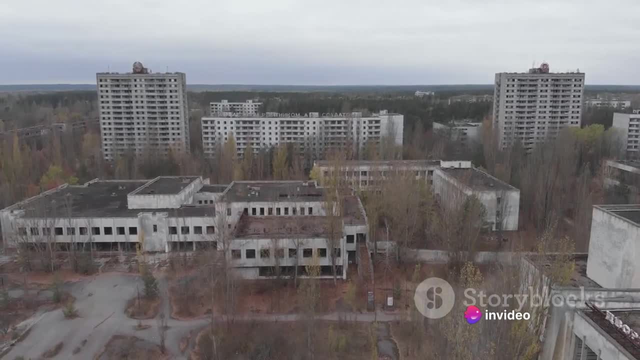 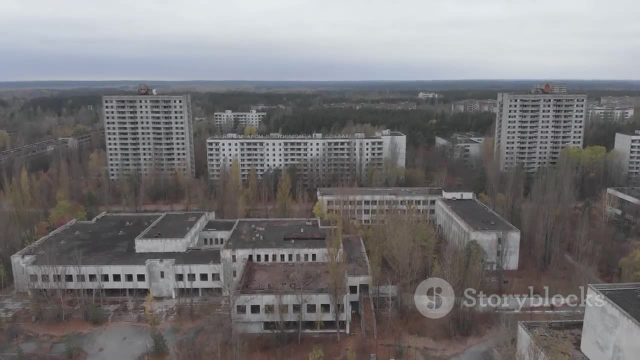 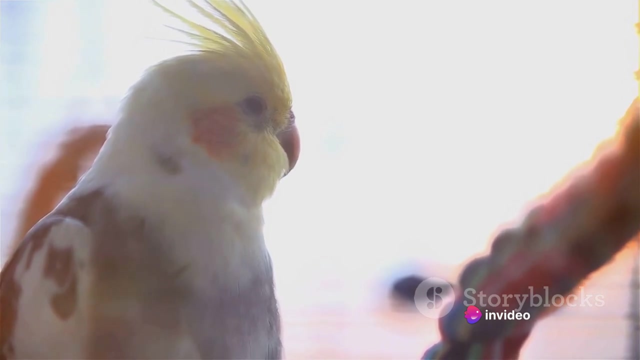 Carolina discovered certain species of birds in Chernobyl, like the great tit, exhibiting signs of genetic changes that enhance their resistance to radiation's harmful effects. On the other hand, Radiation isn't without its adverse effects. Studies have shown that birds exposed to radiation often exhibit physical abnormalities, such as smaller brains and cataracts. 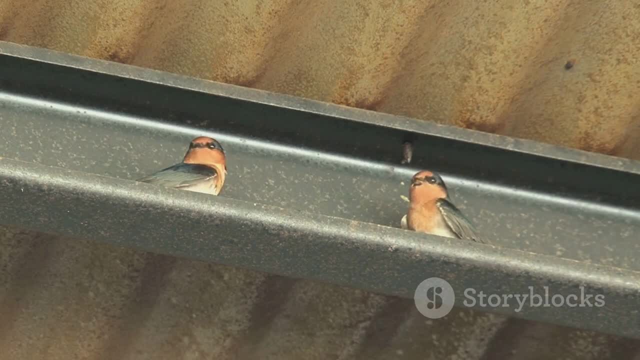 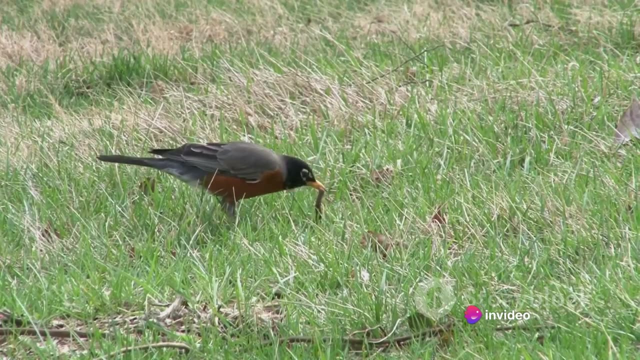 Researchers from the University of Antwerp found that barn swallows living in Chernobyl's radiation zone had a higher frequency of tumors and genetic mutations compared to those in non-radiated areas. Moreover, radiation has been found to impact birds' reproduction. 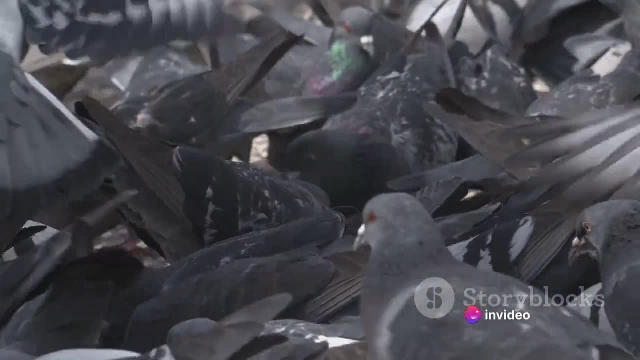 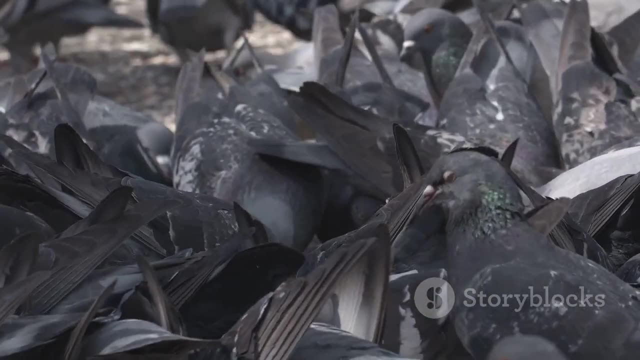 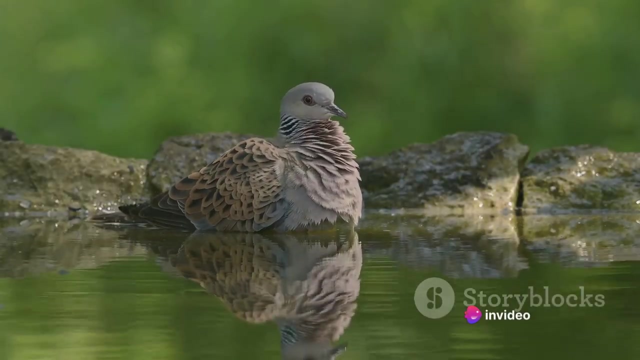 A study from the University of St Andrews revealed that birds in high-radiation areas produced fewer offspring, with some species, like the tree pipit, showing a decline of up to 40% in their population. It's also important to note that the effects of radiation on birds can vary depending on the species and the individual's genetic makeup. 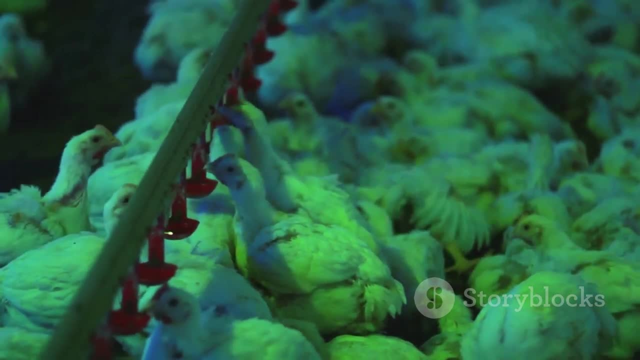 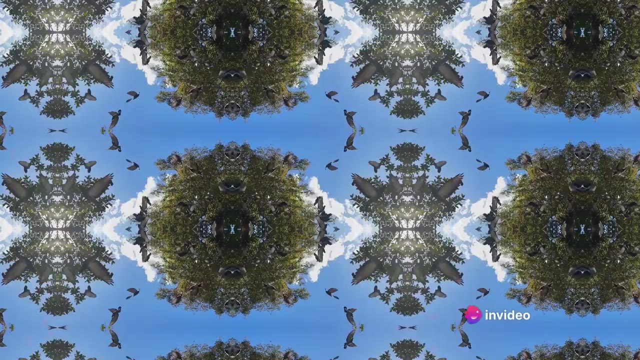 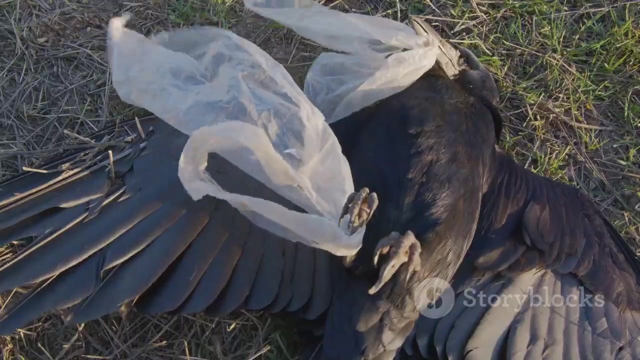 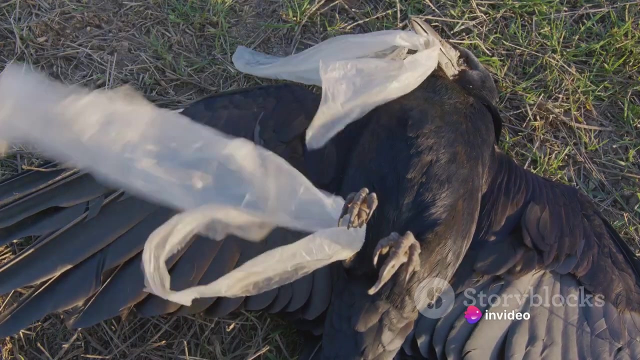 For instance, the oriental turtle dove has shown a surprising resilience to radiation, with populations thriving in areas still considered. In conclusion, the impact of radiation on birds is a complex issue with no black-and-white answers. On one hand, we see evidence of harmful effects, such as physical deformities, genetic mutations and reduced reproduction. 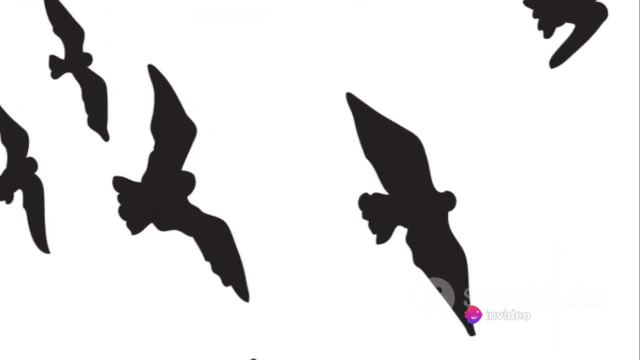 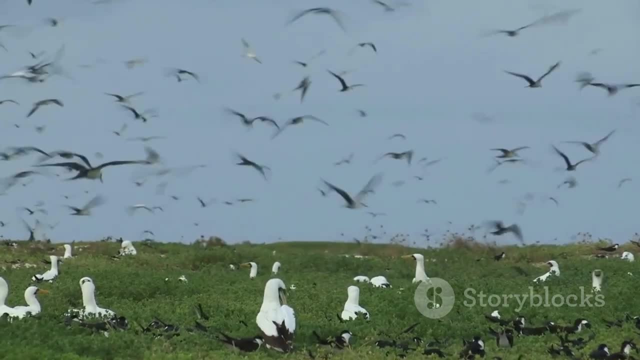 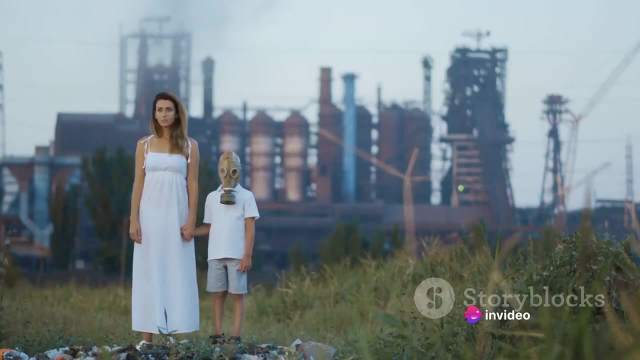 On the other hand, some species show signs of adaptation, developing genetic changes that increase their resistance to radiation. It's a captivating testament to the resilience and adaptability of nature, even in the face of the pandemic. However, it also underscores the importance of minimizing our impact on the environment and preventing future nuclear disasters.